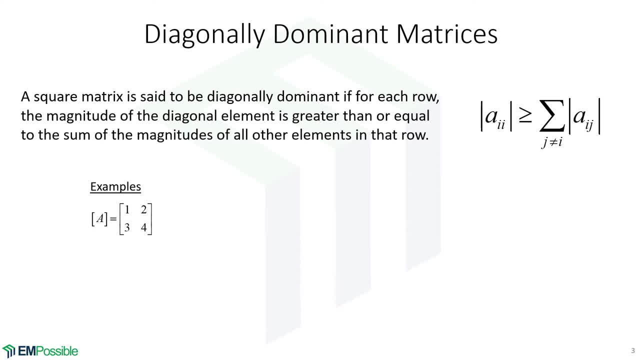 examples: Here's a matrix: one, two, three, four. Is that a diagonally dominant matrix? The answer is no, and that's simply because in the first row our diagonal element one is actually less than two, so that's not diagonally dominant. 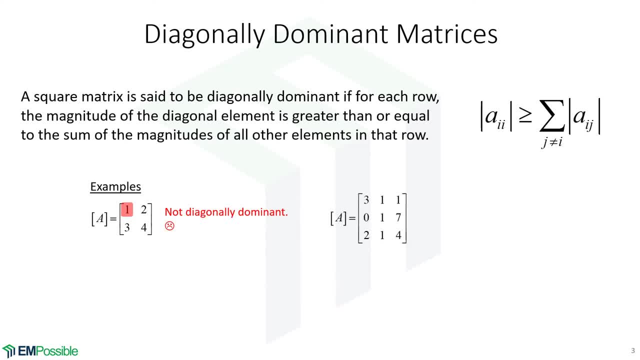 Here's a new matrix. Is this diagonally dominant? This is not diagonally dominant because of the second row. We have a one in this position and that's less than seven over here. How about this matrix? Is this a diagonally dominant matrix? 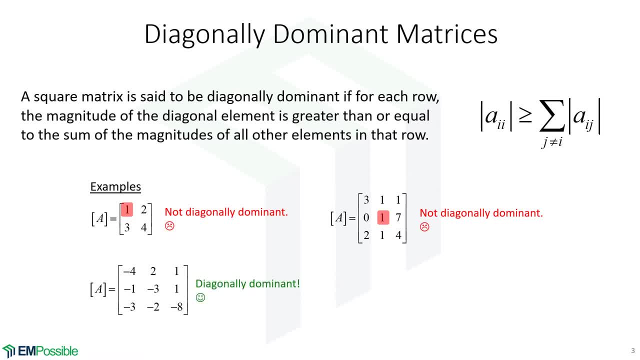 It turns out that is a diagonally dominant matrix. So in our minds, throw out all the negative signs and what we can see is four is definitely greater than two plus one or three. Three is definitely greater than one plus one, which is two and over here, eight is definitely. 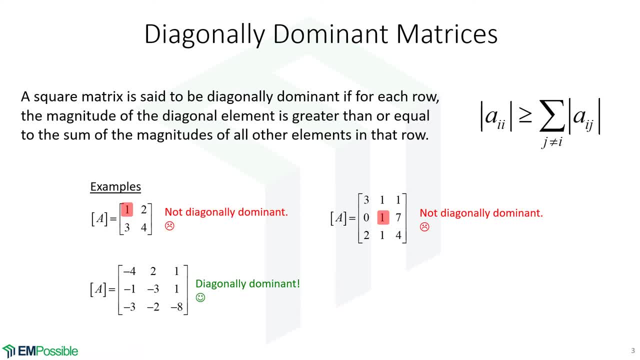 greater than two plus three, which is five. So we have a diagonal element and that's a diagonally dominant matrix. So we have a diagonally dominant matrix, and a matrix like that could be solved with Jacobi iteration. One last example: Is this diagonally dominant And it's no, and that's. 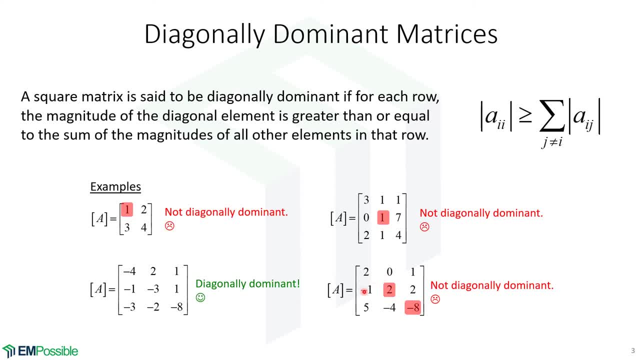 because two is not greater than one plus two, which is three. Likewise, in this row, eight is not greater than four plus five, which is nine. So that is not greater than one plus two, which is nine. So that is not a diagonally dominant matrix and Jacobi iteration probably could not be applied to. 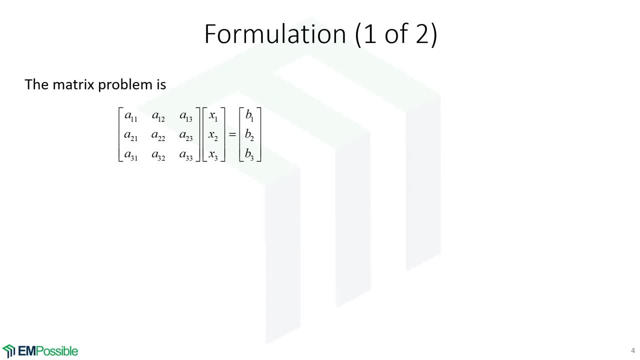 that Let's formulate the Jacobi iteration, and we're going to do this two ways. The first will be purely algebraic and then the second one will come up with a matrix equation. So we're working with matrices instead of the individual terms. So here's our matrix problem that we would like. 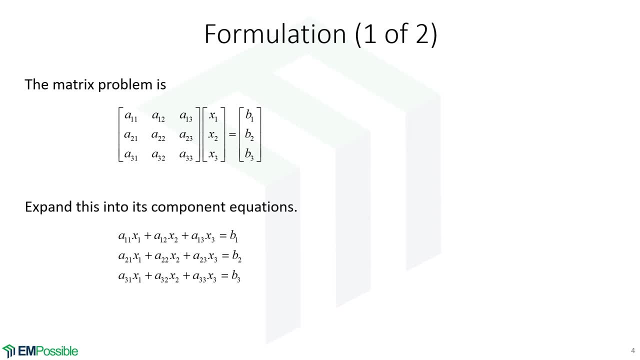 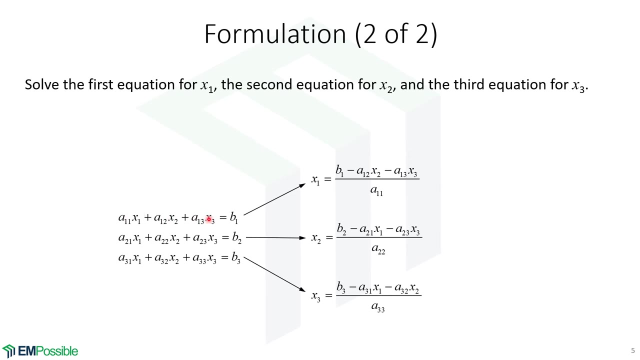 to solve with Jacobi iteration. The first thing we'll do is jump out of matrix form and write this matrix equation as three separate linear algebra equations. Now, from there, what we're going to do is go each row at a time, solve. 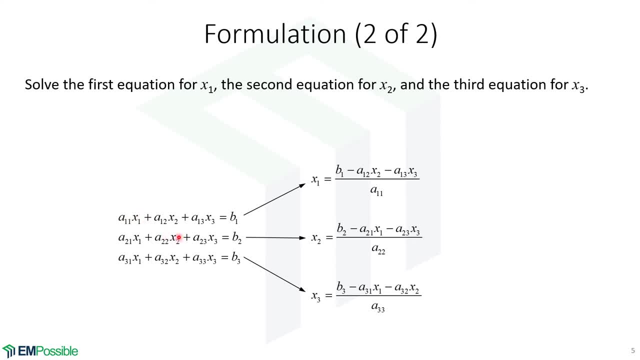 the first row for x1,, solve the second row for x2, and solve the third row for x3.. And that's where we end up. So we have these three equations solved for x1,, x2, and x3.. And it turns out: 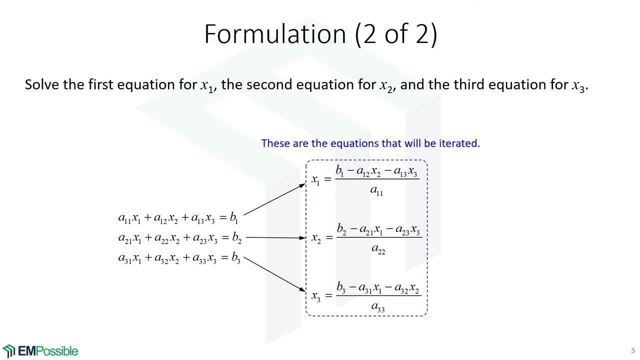 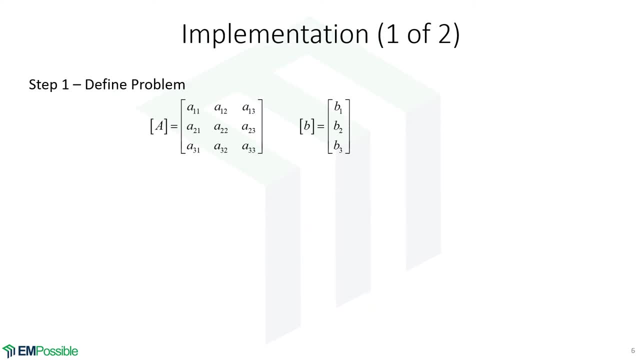 these are going to be the equations that we iterate to improve our guess at x1, x2, x3, every iteration. So here's how we would implement that. Well, we start with the problem. We need our ax equals b. x is what we're trying to find, so we need a and b to begin with. We then come up with: 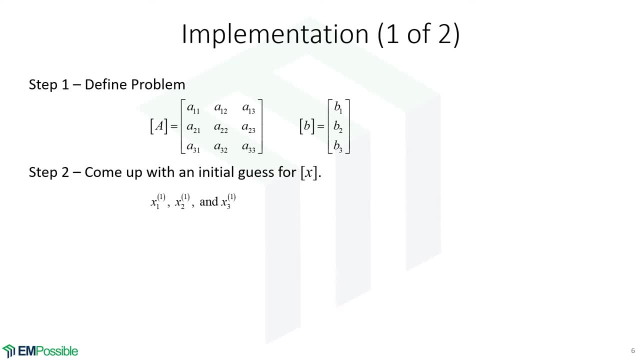 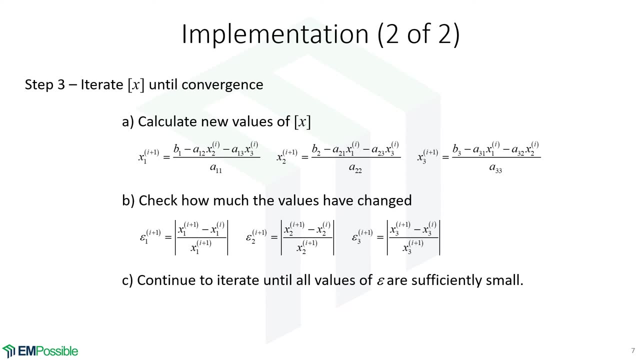 an initial guess, and the better we can do that, the better off we'll be. Now we go into our iteration. So we have this initial guess. The first thing we're going to do is go through these three equations to calculate better values for x1,, x2, and x3. Once we do that, we're going to 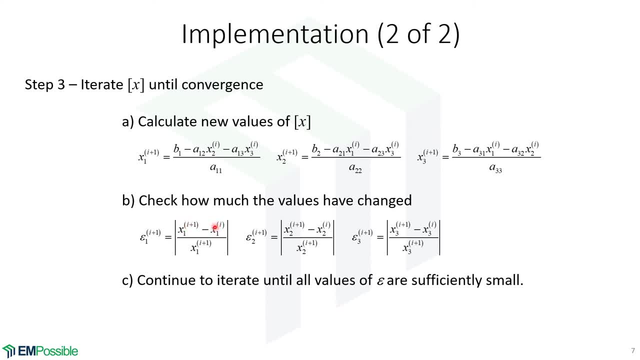 compare what we've just calculated to the previous iteration and of course we'll normalize that to our x value. So we really kind of have percent errors here. So we have an error for x1, an error for x2, an error for x3, and we might add them up, We might look at the largest. 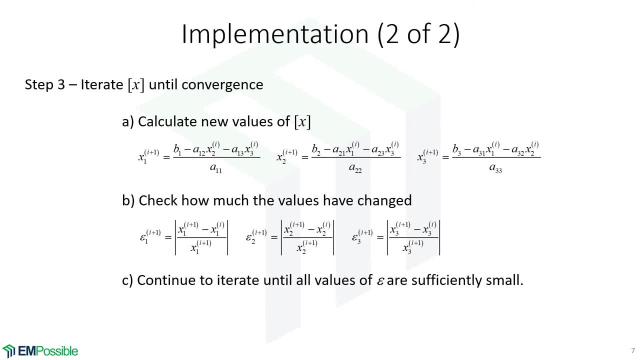 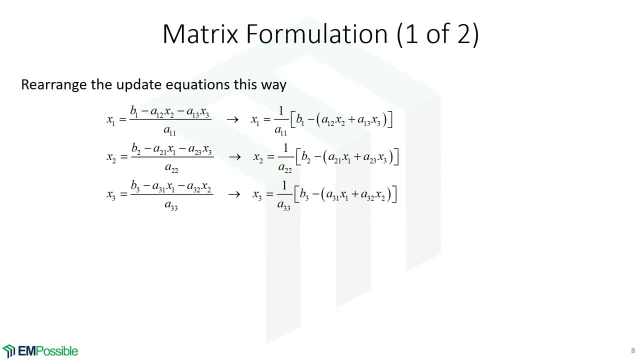 one, but we're going to iterate until all of those errors are sufficiently small, and then we'll have our answer. that's it. let's look at how to do this with matrices, so we don't have these large algebraic equations. the first thing we'll do is we'll look at the equations that we're iterating. 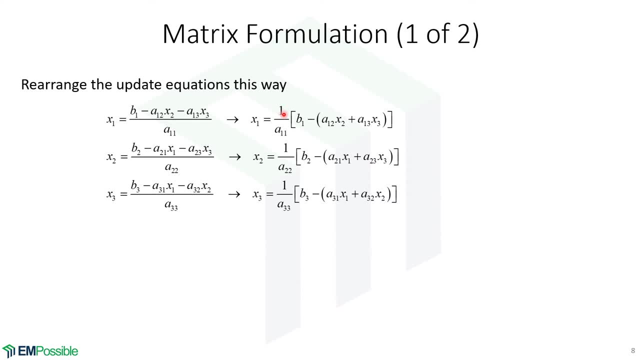 same equations. we're just going to write them slightly differently. so we have this one over a11 and then what was in the numerator? we're writing over here and looking at this form and maybe this takes some practice, but somebody as crazy as me that's been doing this long enough. 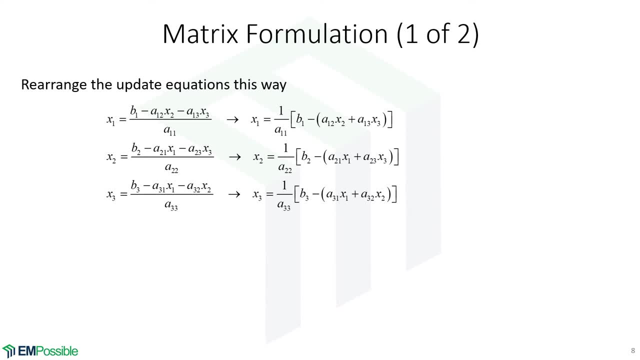 i can look at those and actually write a matrix equation. so i'm looking at the left, i see my x values, so that's a column vector of x's. i then see the diagonal elements of a1 over the diagonal elements of a. so what i'm going to do, 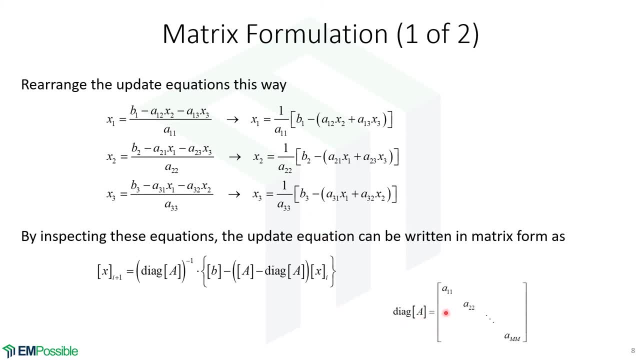 is okay. if we have this operation, diag a, we're going to form a new matrix that essentially just pulls out the diagonal, and matlab has a command, diag, that actually does that. so we're going to take the diagonal out of a and invert that. that's our next matrix. then we're going to multiply a. 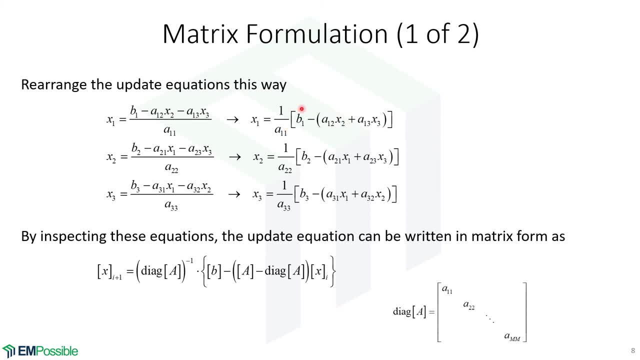 bunch of other stuff which i'm reading off of here. the next thing i'm looking at is all of the b's. this is a column vector, so we have our column vector of b's, so we're going to take the diagonal out of a and invert that. that's our next matrix. then we're. 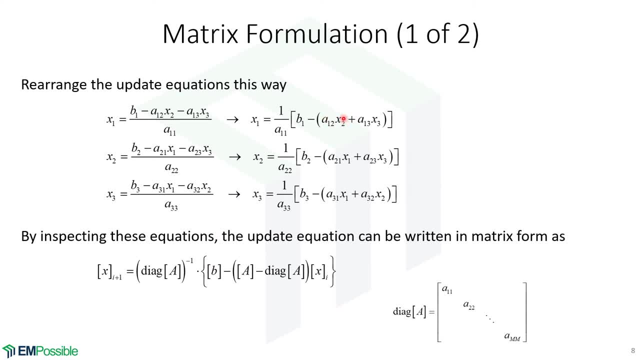 going to take the diagonal out of a and invert that. that's our next matrix. then we're going to. now we have what looks like a times x, right, but it's missing a term in each one. it's missing the diagonal element. we see no a11 times x1 here. we see no a22 times x2 and down. 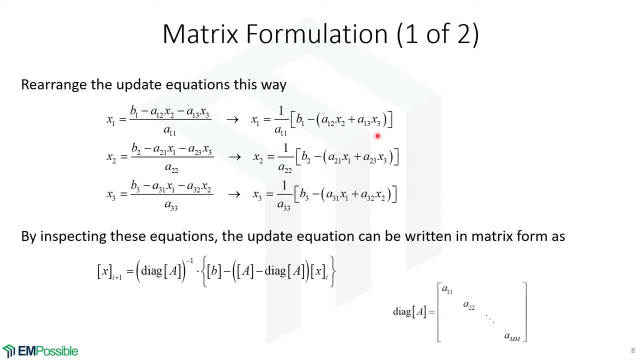 here we see no, a33 times x3. so this is kind of like a times x, but without the diagonal element. so we'll take a, we'll subtract the diagonal of it and put that in parentheses. so that's our new a, without the diagonal, and multiply that by x. 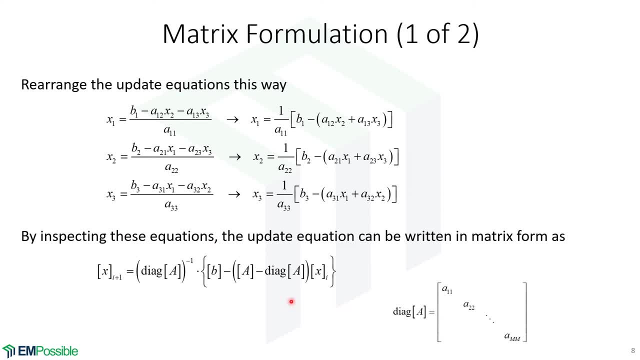 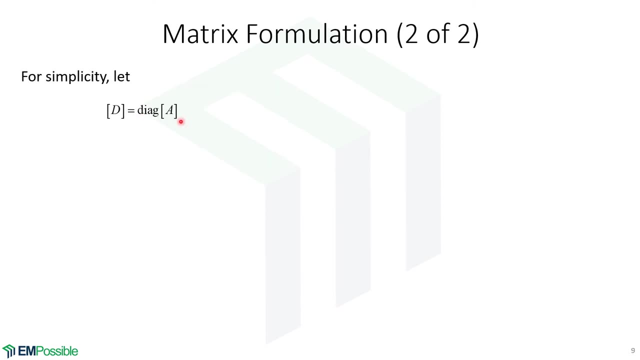 so this is a new matrix equation that we don't have to have. we don't have to track all of these separate equations, and this is really valid for any number of equations. our matrix might be 10 000 by 10 000.. let's keep going for simplicity. let's not keep writing diag of a. let's just call that d. 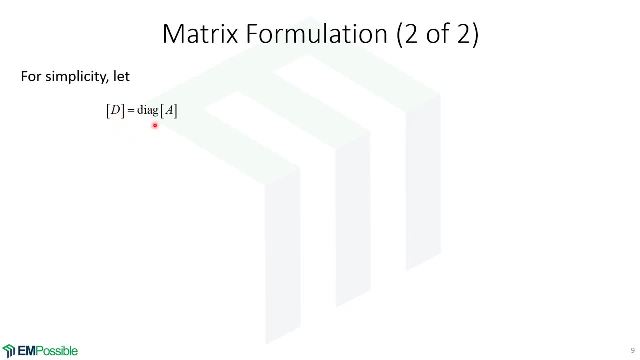 so we'll remember, d is a diagonal matrix which is the center diagonal of a. so that means the equation we derived on the previous slide is: inverse of d times all this stuff, so column vector b minus, and then, in parentheses, a minus d, that stuff, in parentheses, times column vector a. so this is our x from a, our current iteration. 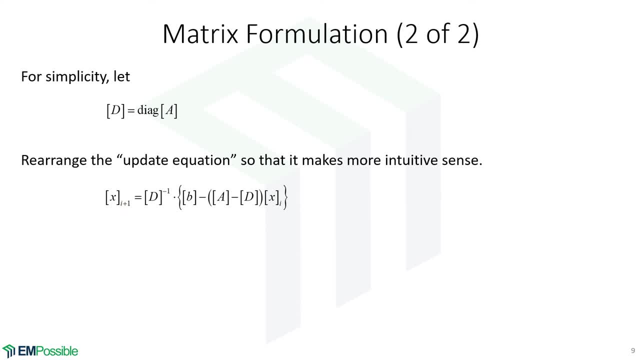 and from all this we calculate x. at the next iteration we're going to do some algebra on this. to put it in a slightly different form, the first thing we'll do is just multiply everything out. we got a bunch of stuff to multiply out. we have you know what's in parentheses here with this x, and then we have this d inverse. we're going to 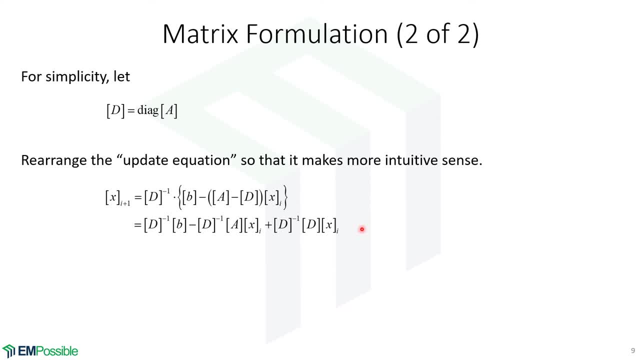 multiply everything out and that's where we end up. and we can simplify this a little bit. we see a d inverse, d, right, that's the identity matrix, and identity matrix times column vector x. that's just column vector x, so we can write this as just that column vector x plus everything else. so 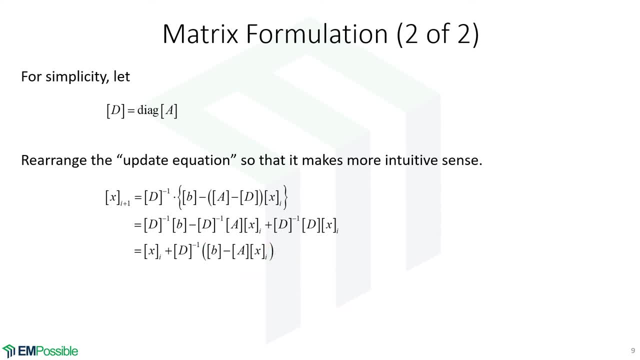 we simplified everything else down to a, a smaller term. we still have one of our x's left, so that's. we just leave that there. that came from here. so here's our new form of the equation. now it turns out so column vector x at iteration i plus 1 is going to equal this, and we can look at this and: 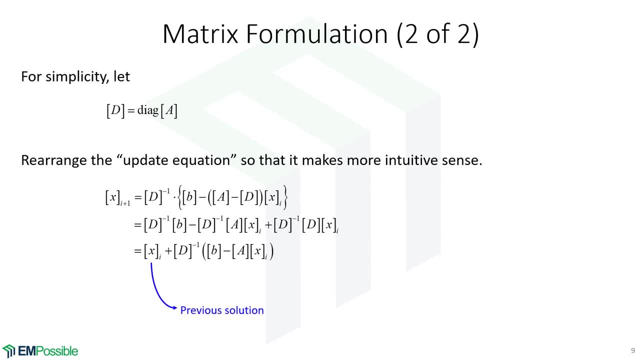 interpret that a little bit physically. so this first term is the x from the previous iteration, which means whatever is left over is the improvement on x. and that's very useful because then we can look at the magnitude of that improvement to determine if our iterations have converged. if that improvement becomes sufficiently small, we can say that we're done. 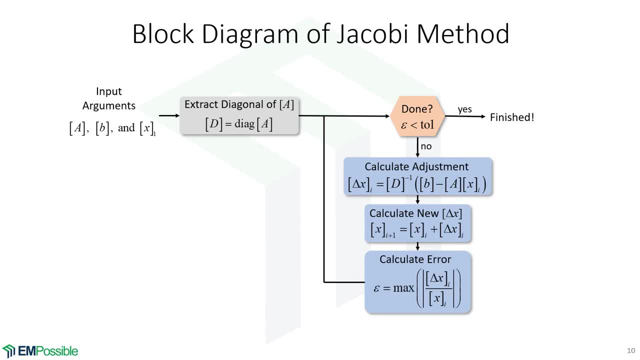 so here's the algorithm of the jacobi method. so we start with, of course, a and b. that's the matrix problem we're trying to solve and a good guess. if we don't have a good guess, maybe we just put random numbers in here or whatever. but hopefully we have a good guess. step one: we will pull the diagonal out of a and just 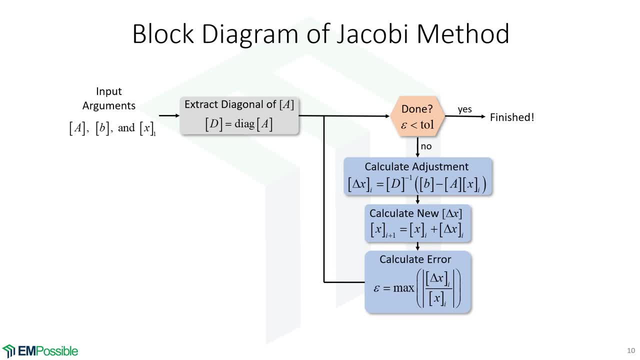 call that d. now we enter our our loop and the first thing we'll do is we'll check if we're done- and of course we're not done because we just started, so let's go on. the first thing i'll do is calculate the adjustment. this is how much we have to change our current guess at x to improve. 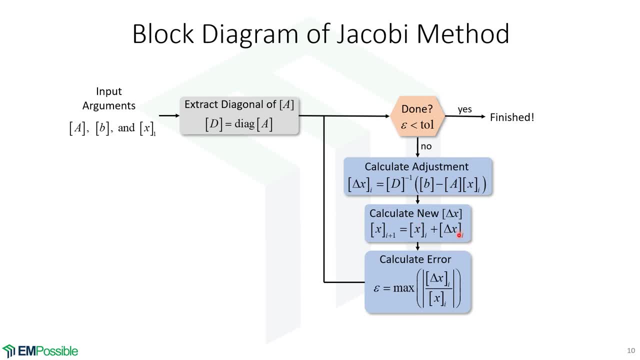 it. then we'll go ahead and prove it. we'll add in that delta x to the previous x to get the new x. but having calculated delta x separately, that lets us check for convergence. we'll take those delta x's by our x's, so we're essentially normalizing it to get percent error and we'll look at the maximum. 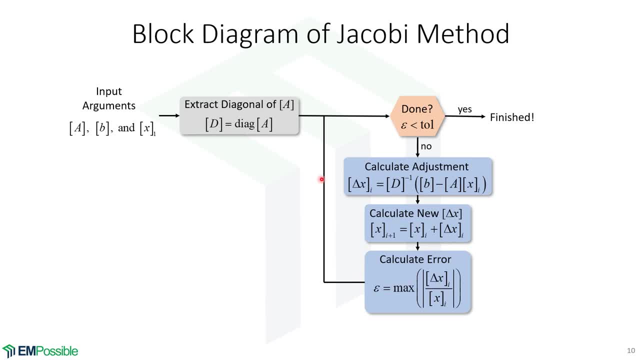 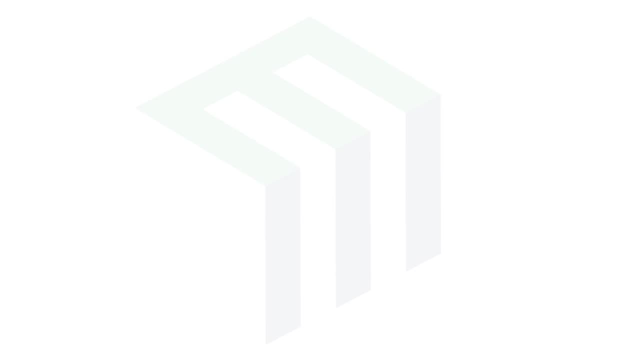 one, the biggest jump, and we'll call that the error and that's what we'll check. when that maximum error for all the variables trying to find falls below some tolerance, we'll say that we're finished and that's it. that's the jacobi method. from the bottom of my heart, thank you very much for watching this video. i love hearing your